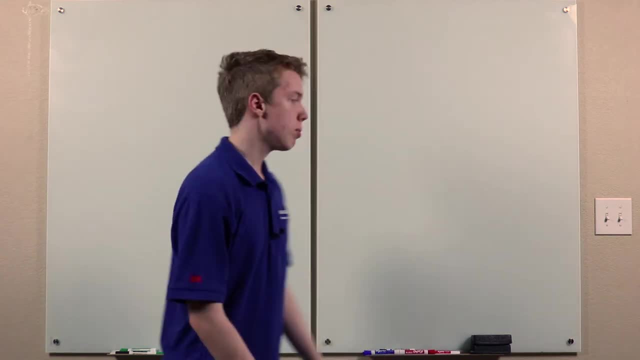 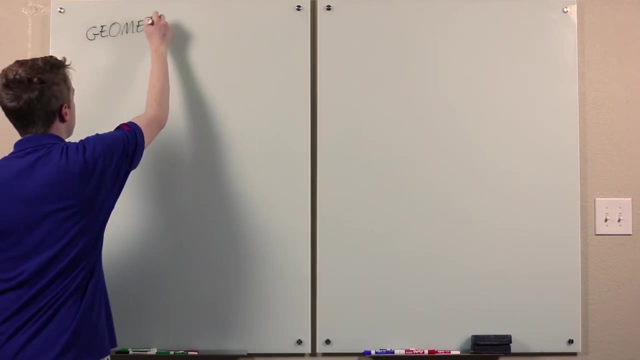 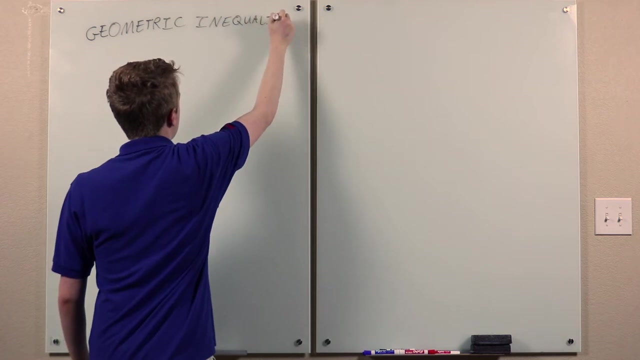 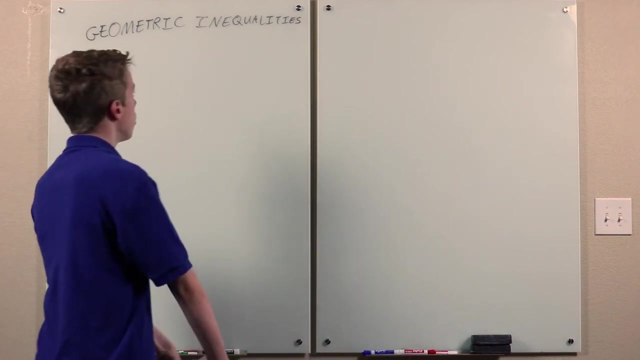 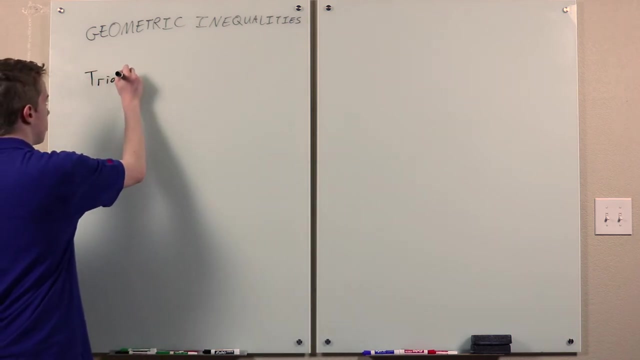 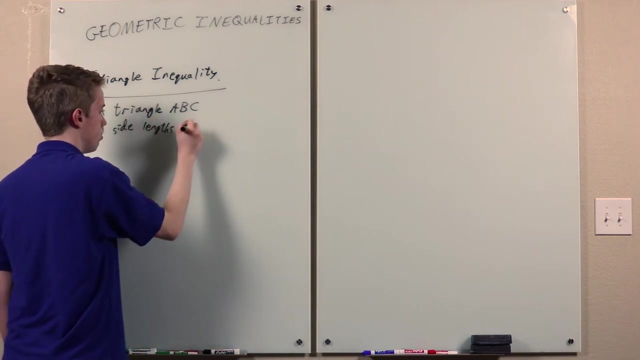 Hi, I'm Luke Robitaille. Let's talk about geometric inequalities. So the most fundamental geometric inequality is the triangle inequality Which is in a triangle, ABC, with side lengths: BC is lowercase a, CA is lowercase b, AB is lowercase c. 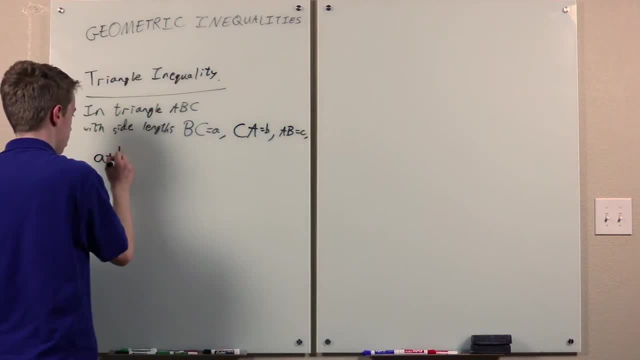 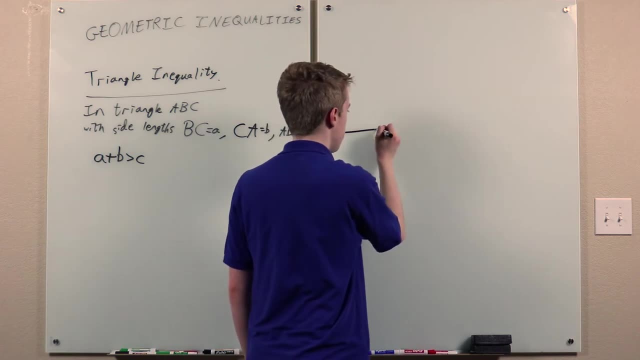 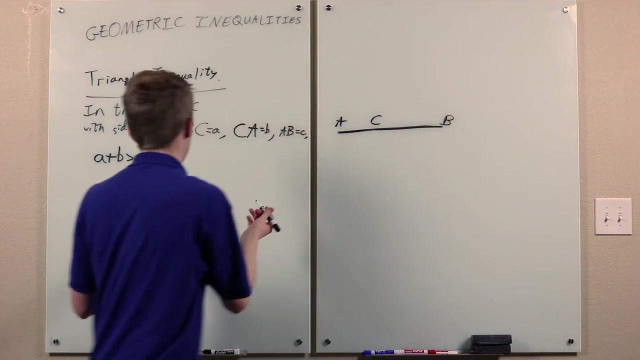 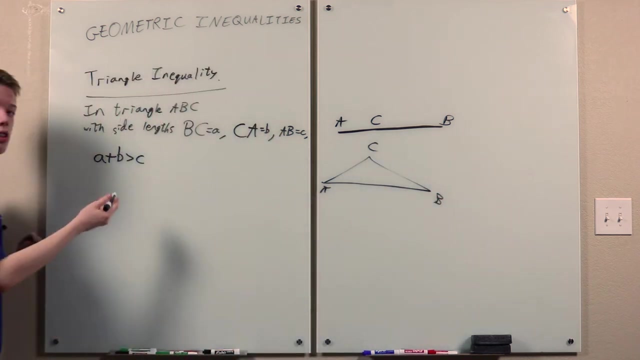 And we're assuming this is an actual triangle. So if it's something like this, where all the vertices are collinear, then that doesn't work. But in a real triangle like this, say, that works. Which basically says the shortest distance between two points is a line segment. 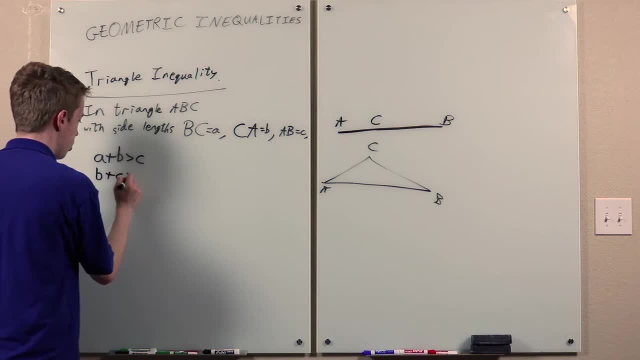 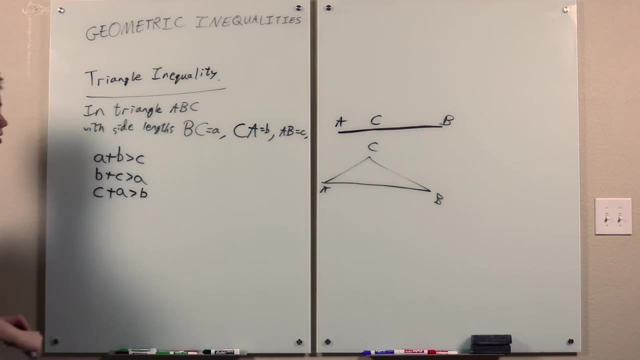 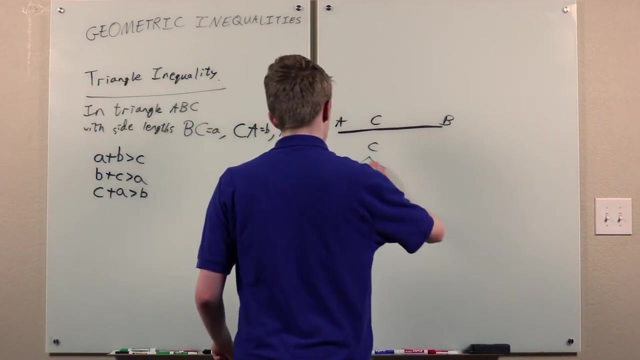 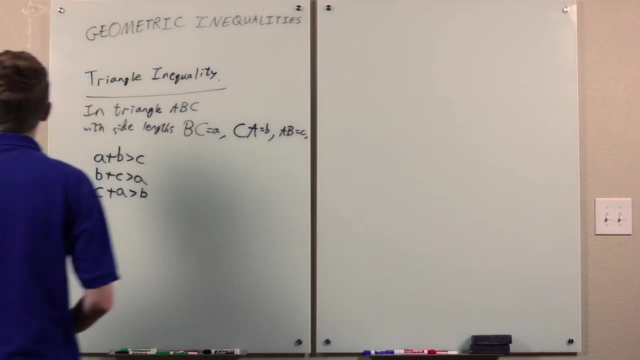 And this is a line segment, And symmetric permutations of this also hold. So we also have this. So a plus b is greater than c, b plus c is greater than a, c plus a is greater than b. And now we have another very important inequality. 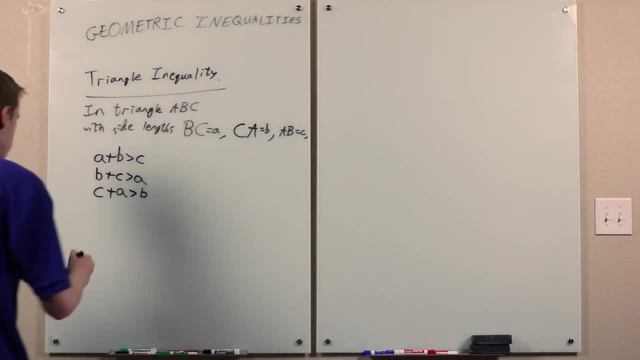 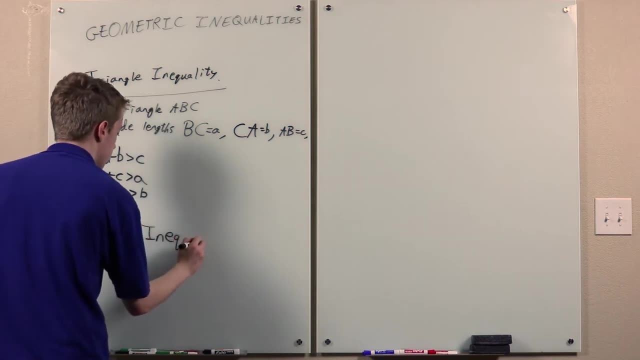 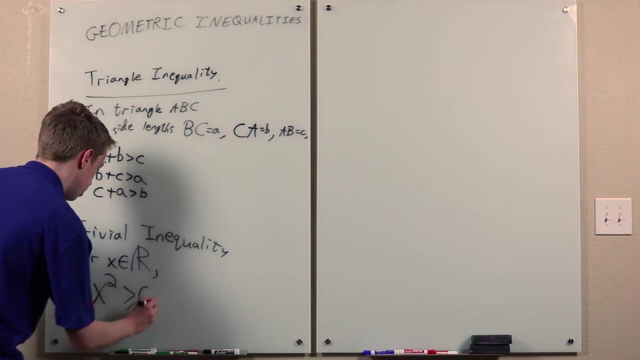 Not strictly a geometric inequality, But it's called the trivial inequality. This is the actual name of this inequality. It says for a real number, x, x, an element of the set of real numbers, X squared is greater than or equal to zero. with equality. 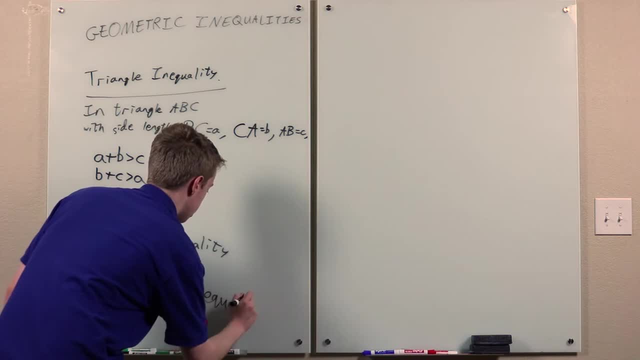 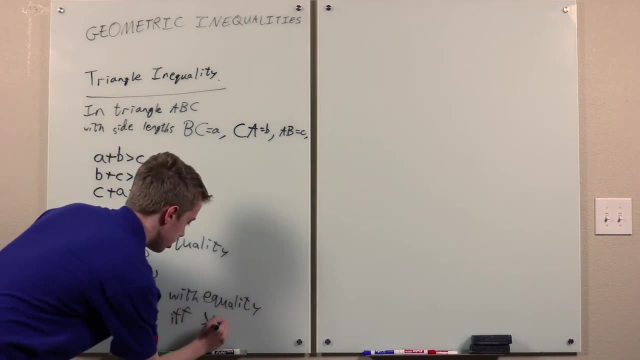 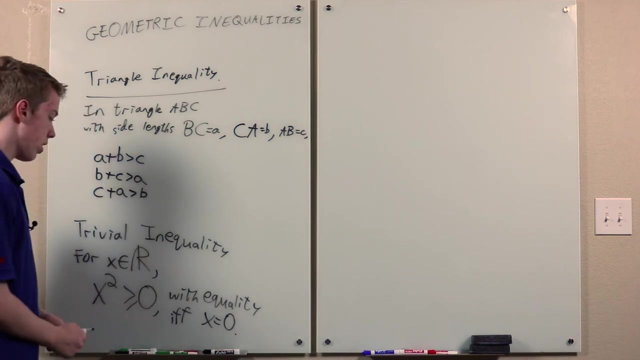 If, and only if. So we abbreviate this by if x equals zero, Not too hard to prove. If x is zero, then we obviously have inequality. I mean, we obviously have equality. If x is positive, then x squared is positive. 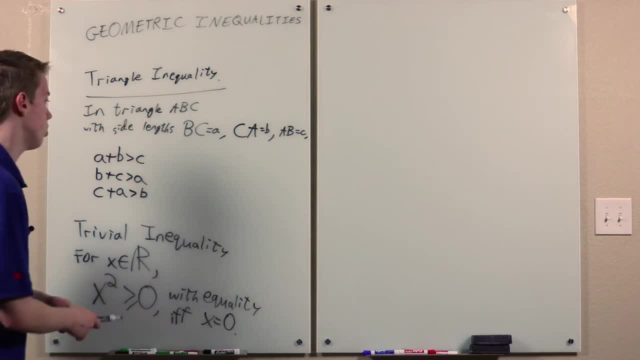 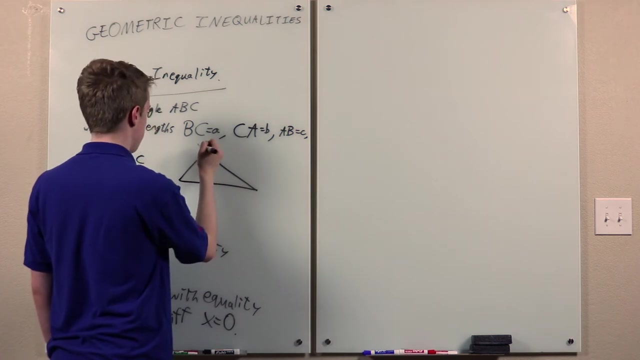 If x is negative, then x squared is positive. So that's why this is true, The triangle inequality: I guess it, maybe I, I guess I should prove it. So basically, we, what we can do, is say and then drop a perpendicular. 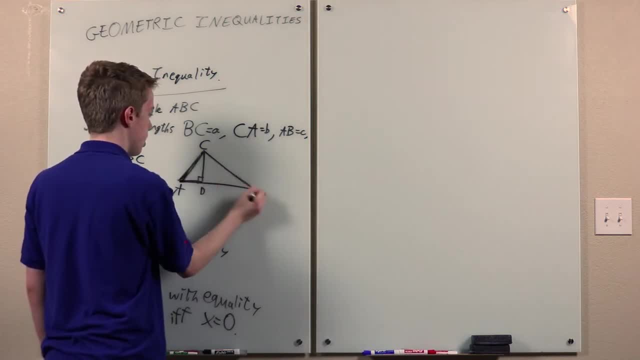 So then a c is greater than a d And c b is greater than d b By the Pythagorean theorem, And then the sum of these is a, b Or, correctly, we could have a diagram that looks like this: 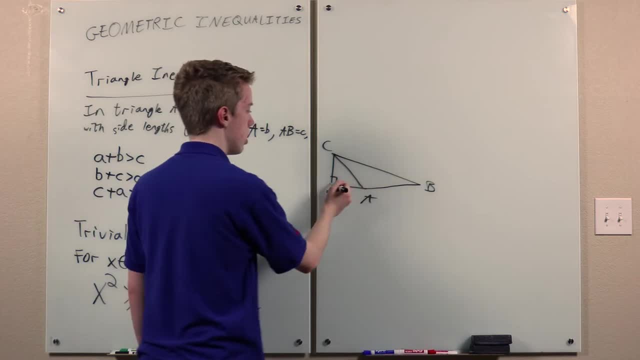 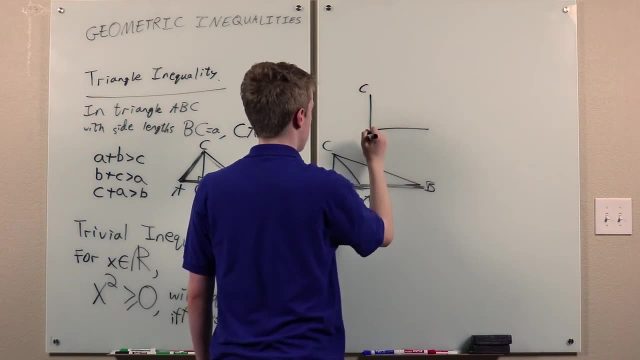 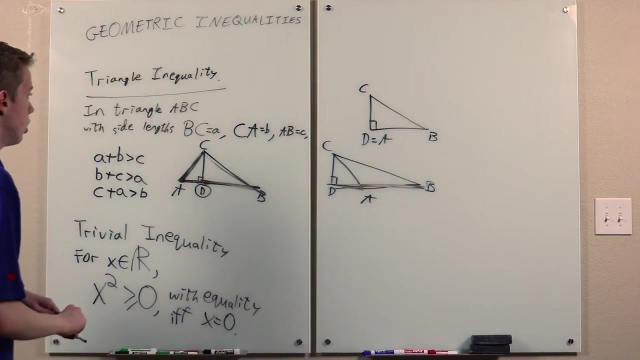 In which case the sum of the lengths is greater than the sum of these lengths is greater than a, b, Or it could be again equal if it's a right triangle. So, yes, that's the triangle, inequality So- and I guess it would be more correct to state it as: 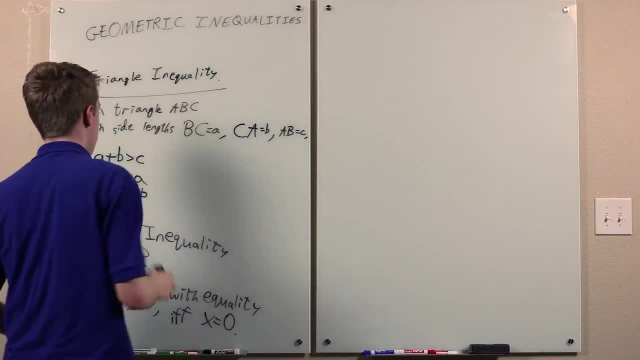 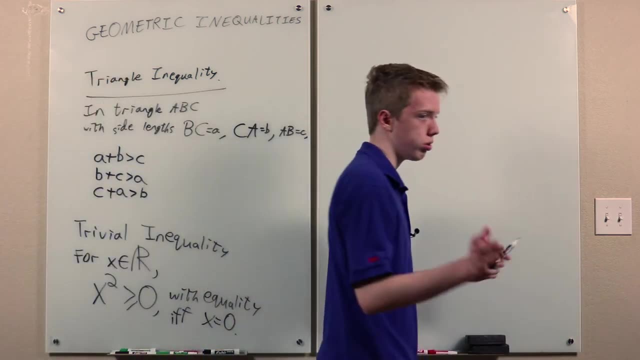 for any points a, b and c. a, b is greater than or equal to c, with equality if, and only if, the point is greater than or equal to c. The point c lies on the segment a- b, So both of those I can call the triangle inequality. 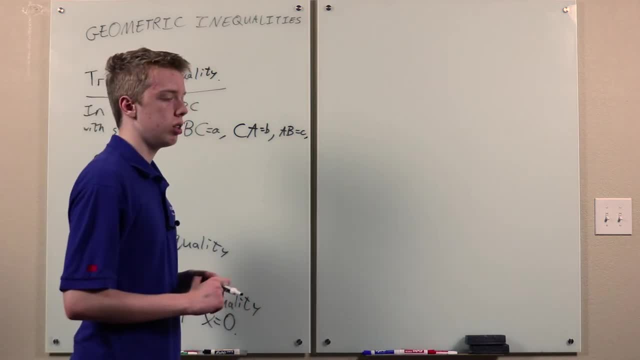 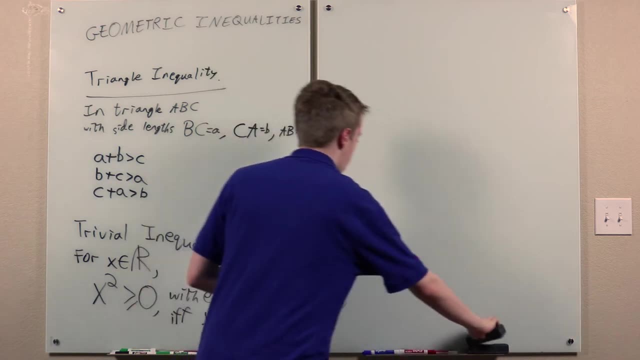 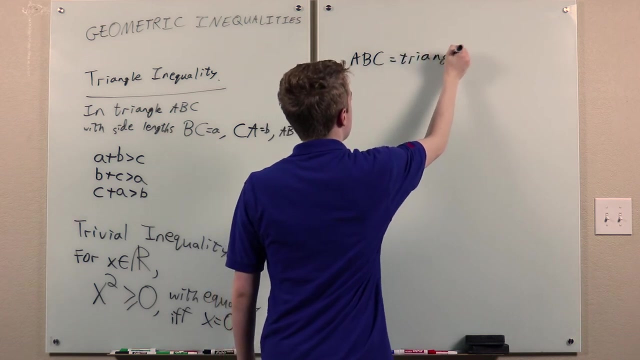 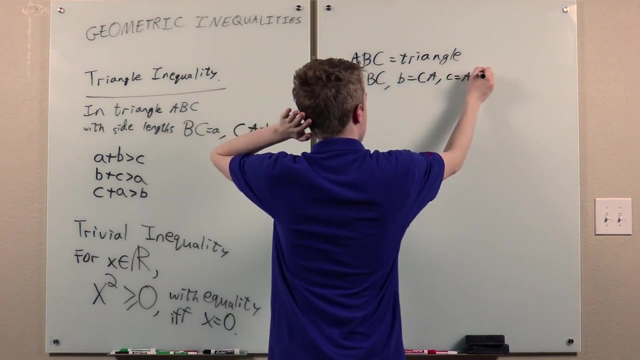 Now let's actually move on to something a little more interesting. So there are several inequalities pertaining to just any arbitrary triangle. So let a, b, c be a triangle, a, b and c be the same And c be the side lengths. 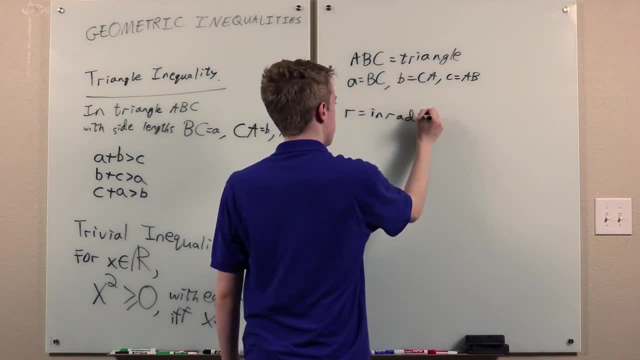 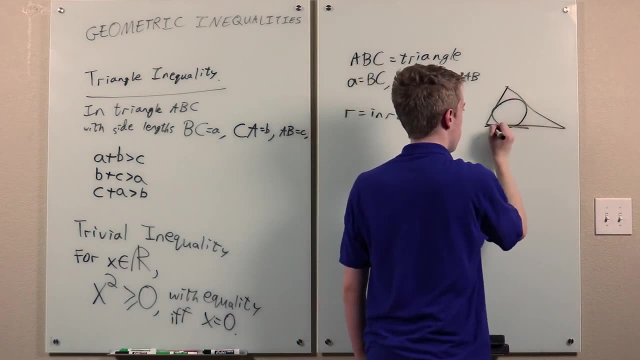 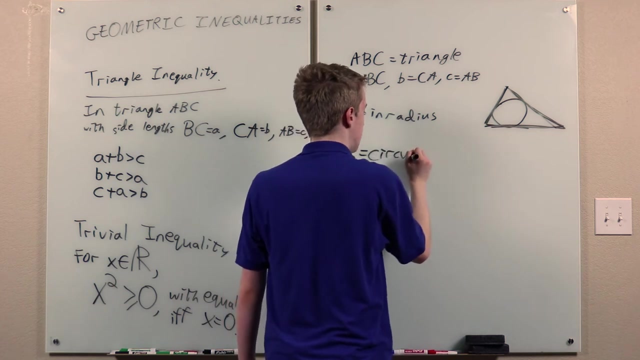 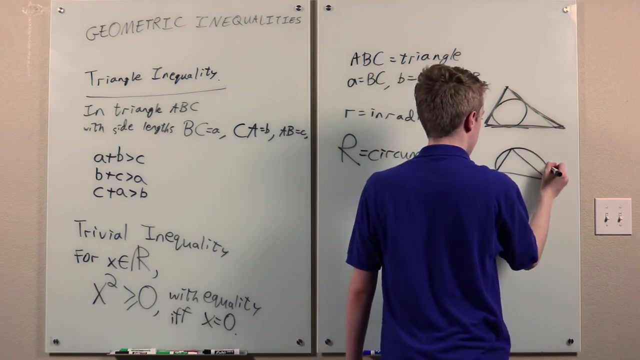 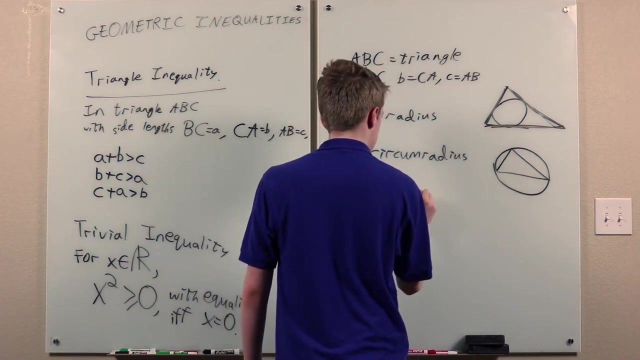 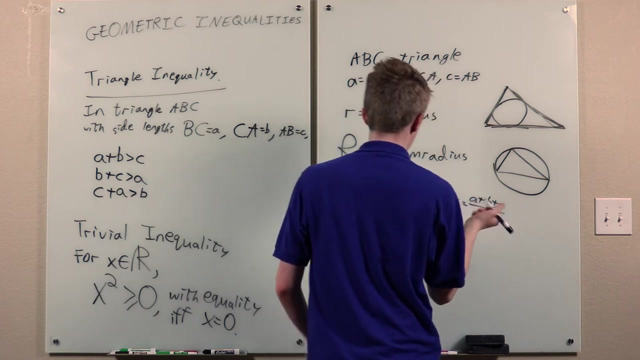 Let r be the in-radius, which is the radius of the inscribed circle tangent to all three sides. Let capital R be the circumradius, the circle passing through all three vertices, And let S be the semi-perimeter, which is the perimeter divided by two. 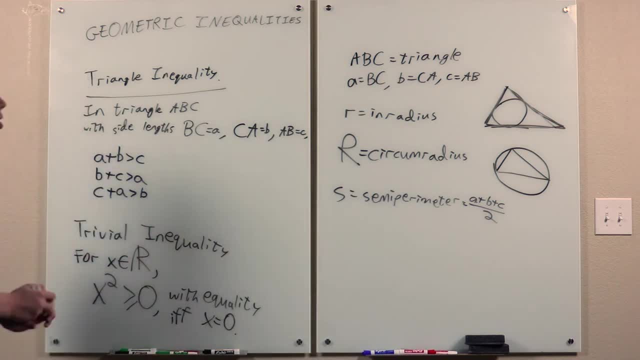 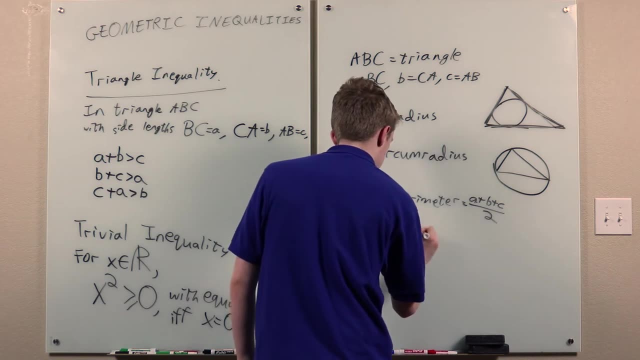 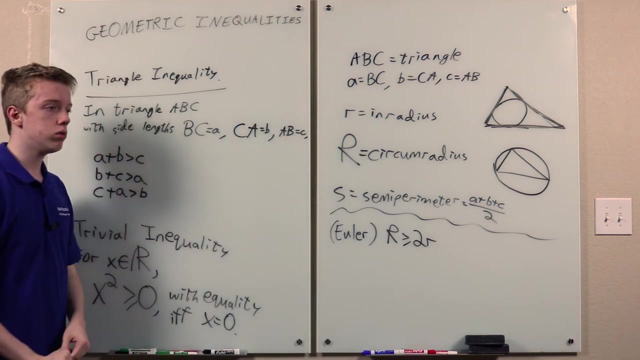 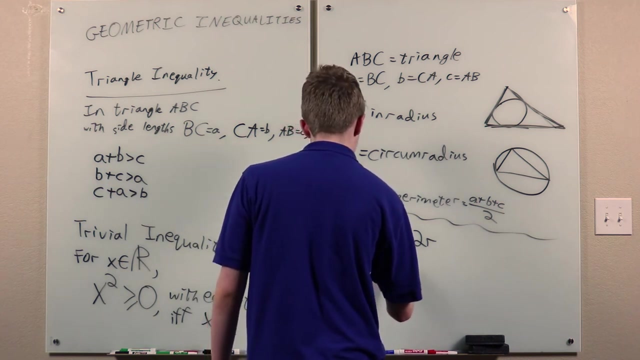 Then we have this famous inequality of Euler, which says that the circumradius is at least twice the in-radius, And then the classical proof. there are other proofs, but the classical proof is to say: this is to prove this, And then appeal to the trivial inequality. 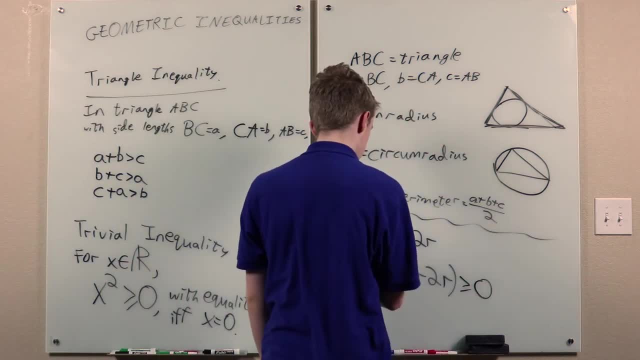 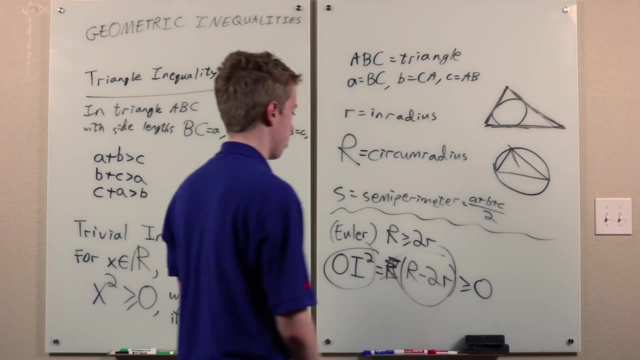 to say now that this is greater than or equal to 0, because this is greater than or equal to 0. And then r is positive, since it's an actual length of something. so then this is non-negative And furthermore, this would give us that equality holds. 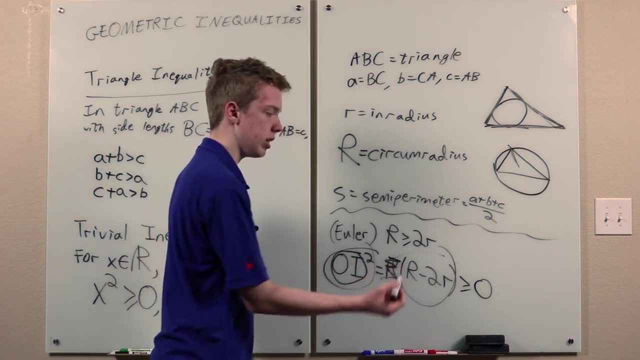 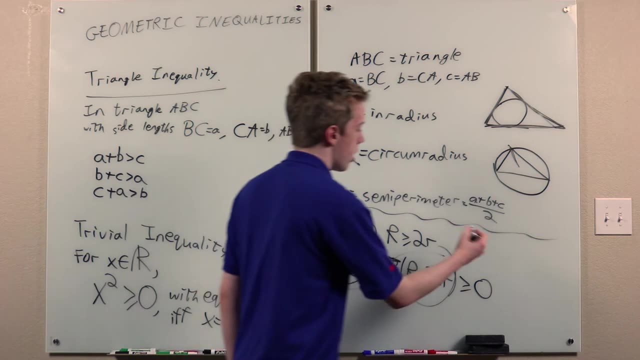 if, and only if, this is 0,, which would mean that the circumcenter is the incenter, which can easily be seen to imply that the triangle ABC is equilateral, And we can verify that we do in fact have equality in that case. 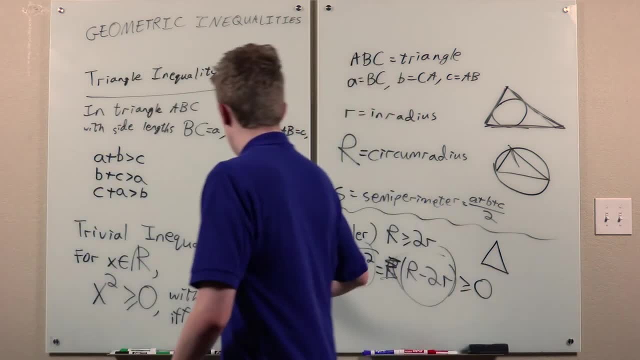 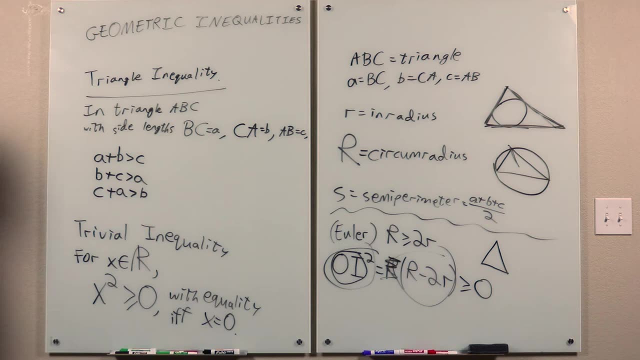 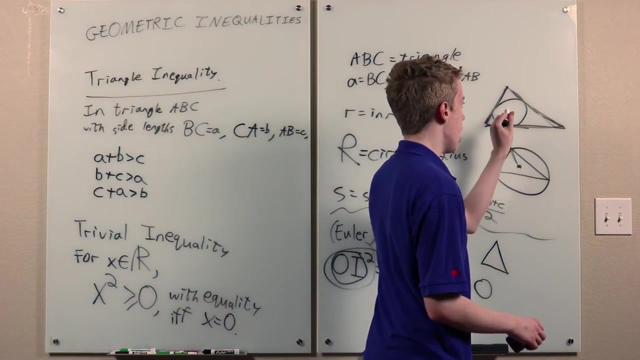 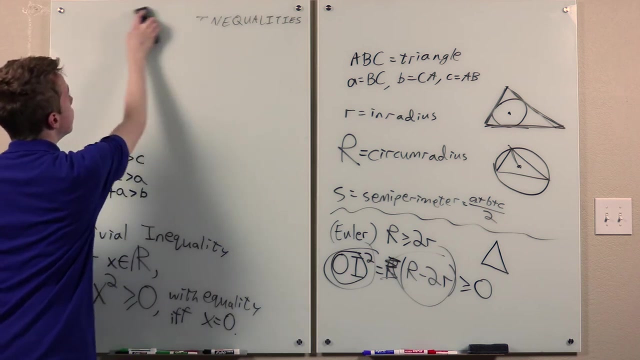 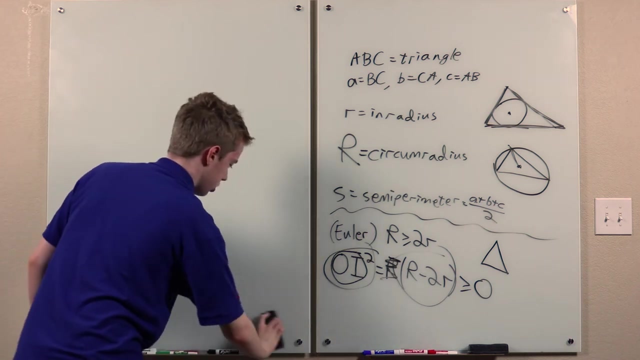 So I'll take a moment to actually prove this statement that OI squared equals r times r minus 2r. Oh, and in this we: O is the circumcenter, the center of the circumcircle, and I is the incenter, the center of the incircle. 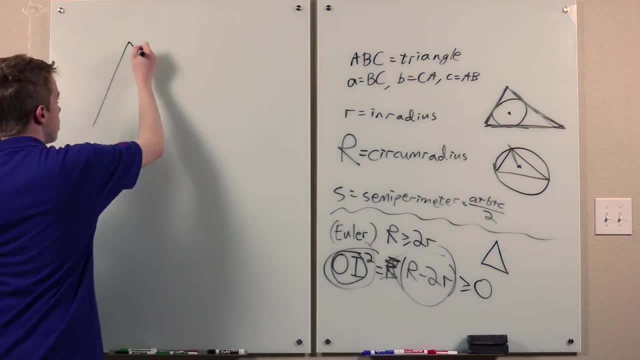 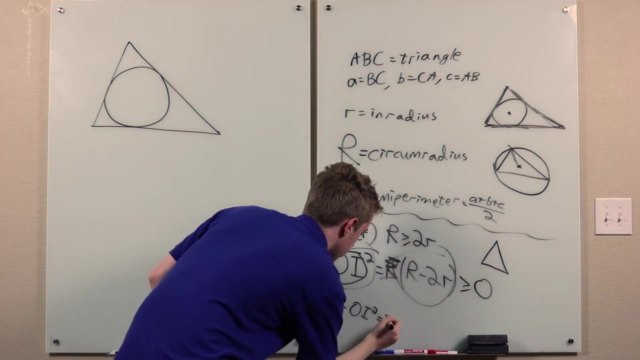 So here's an interesting proof I came up with, And there are many other ways to prove it. There's a more standard proof where we notice that this is equivalent to this, And then we prove that Ai times Id is 2rr because of power of a point. 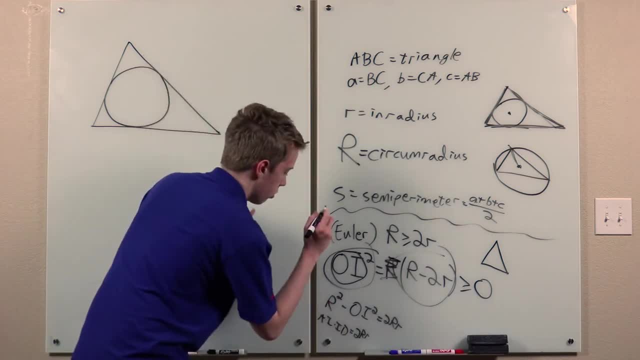 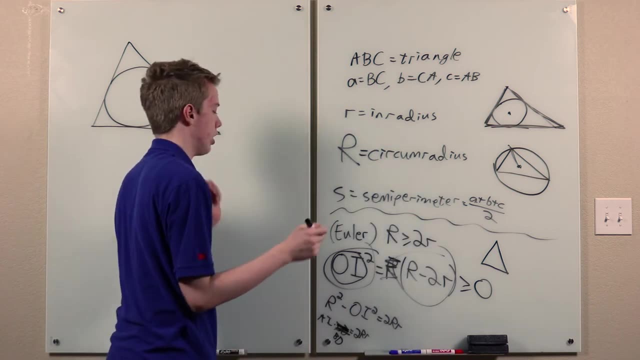 where d is the arc midpoint By the so-called fact 5, this is Bd, where d is the midpoint of minor arc BC of the circumcircle or arc BC not containing a of the circumcircle. And then we write this as this: 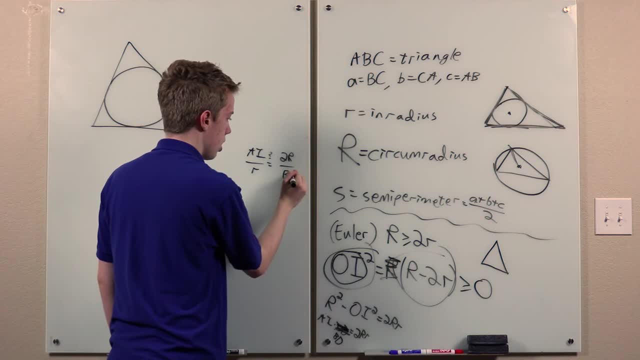 which is what we want to prove, And find a pair of similar right triangles which would look like this: Ai and tangency point to minor arc midpoint, B and major arc midpoint, And this is Bd, this is 2r, this is r and this is Ai. 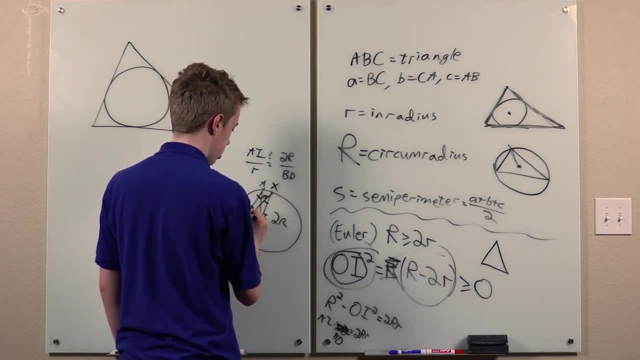 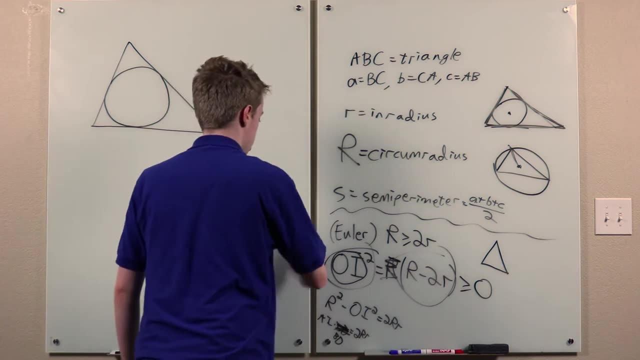 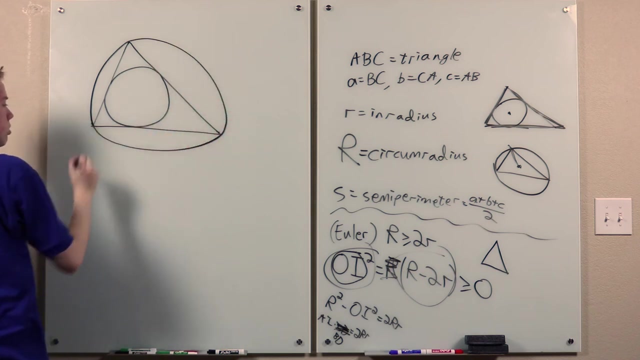 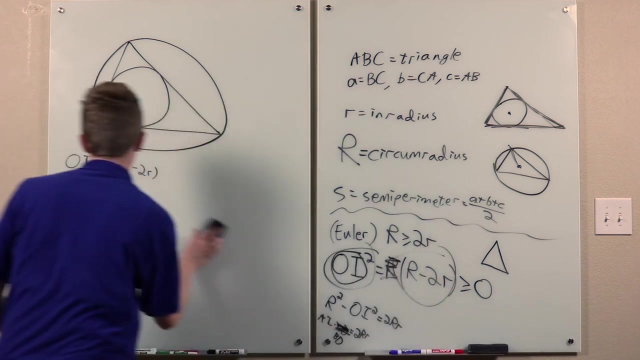 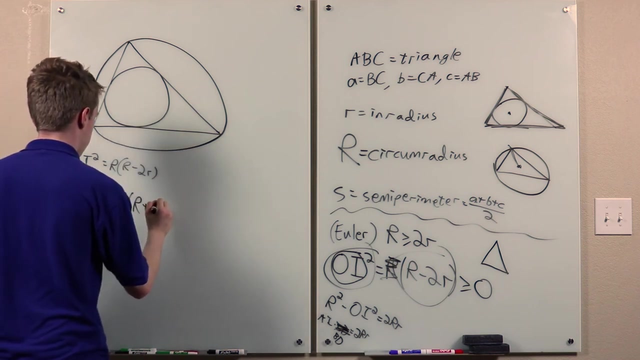 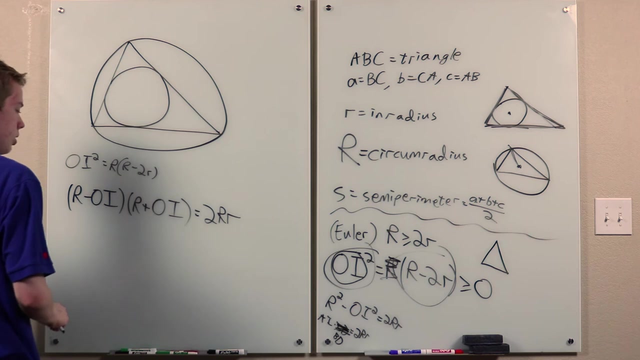 and these angles are right, and this angle is this angle, which is this. Details left as exercise, But instead I want to present a different proof. Here's something that I thought of. So this is equivalent to this, to this, No other way. 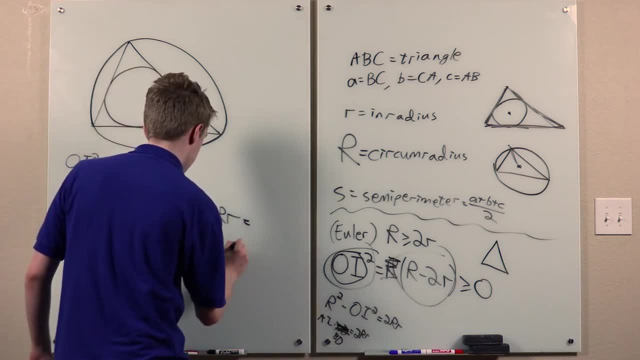 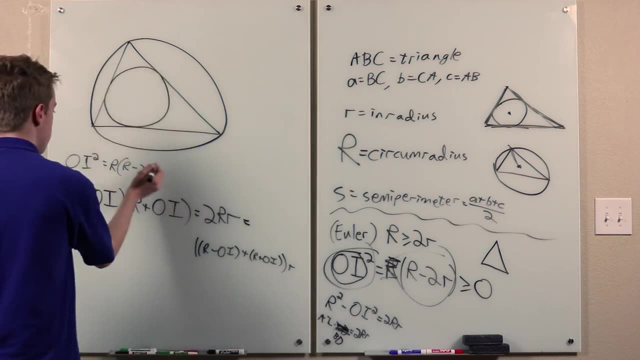 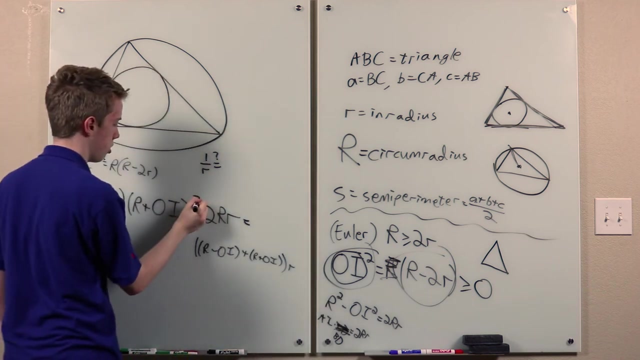 And now we notice that the 2r term is r minus oi plus r plus oi. So we can rewrite the thing that we want to prove as this, And I write a question mark over the equal sign to say that this is what we want to prove. 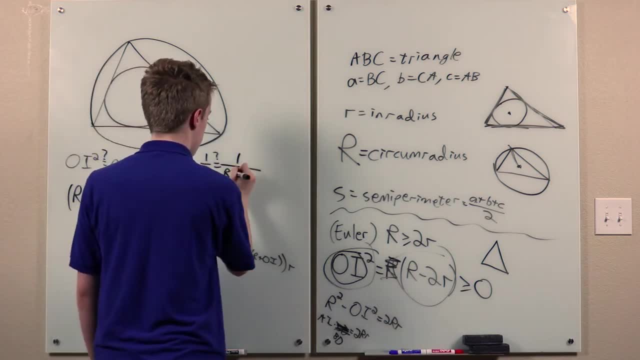 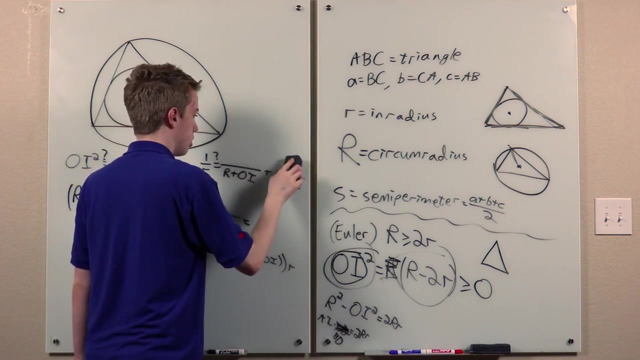 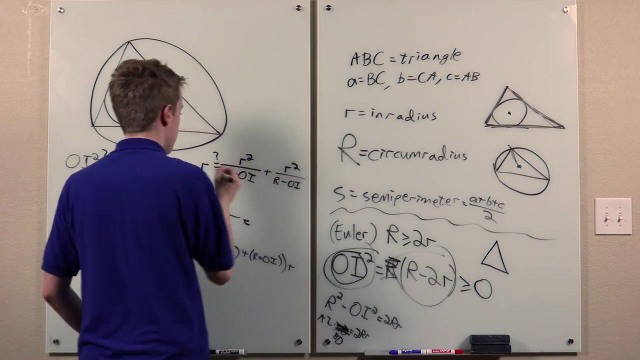 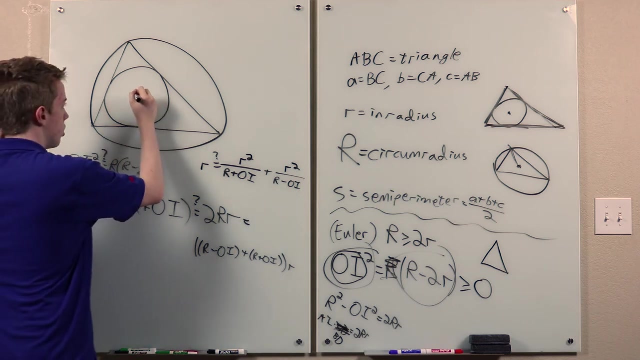 We can write it as: 1 over r equals r over r plus oi, plus 1 over r minus oi. Now let's multiply both sides by r squared, its equivalent, to get that this is what we want to prove. So this suggests inversion. about the in-circle: 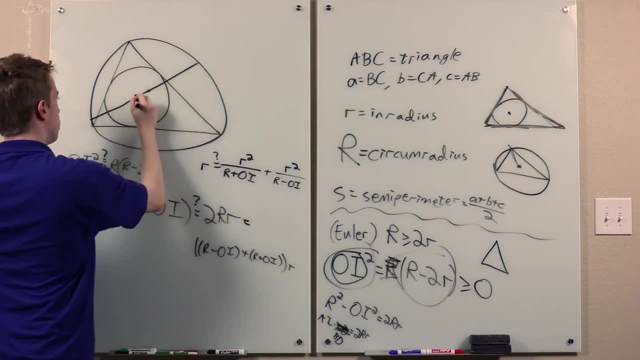 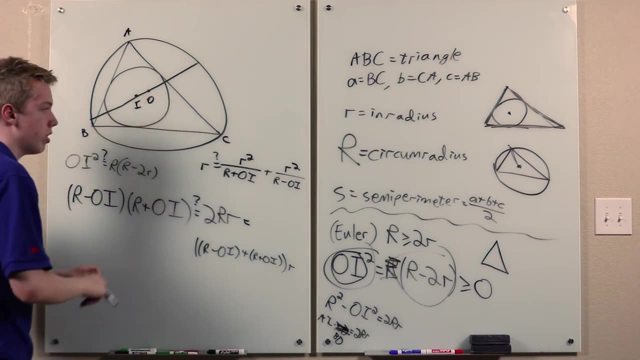 So yes, if o equals i, then the triangle must be equilateral, And then r we can. it's easily computable that this is r plus that r equals big, r equals too little r. so this is trivial. 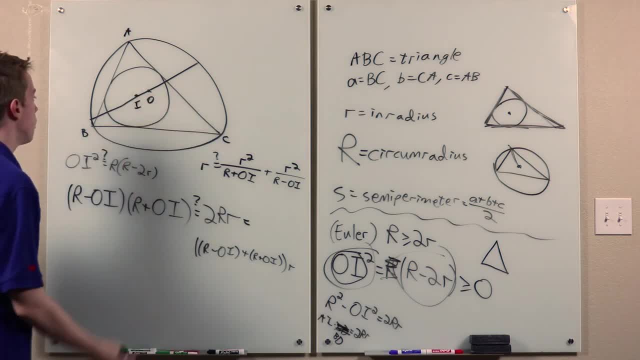 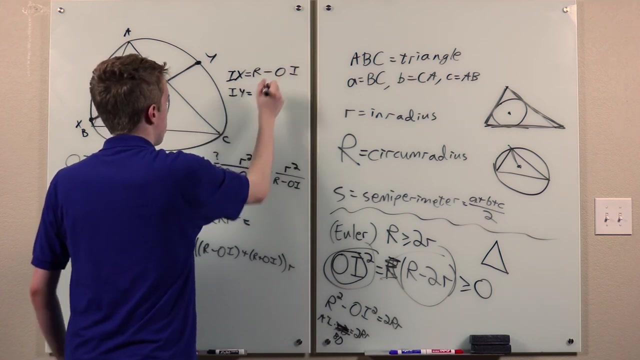 So let's assume that these are two different points. So draw this line oi to intersect the circumcircles at two points, x and y, such that i lies on segment ox. Then ix equals r minus oi and iy equals r plus oi. 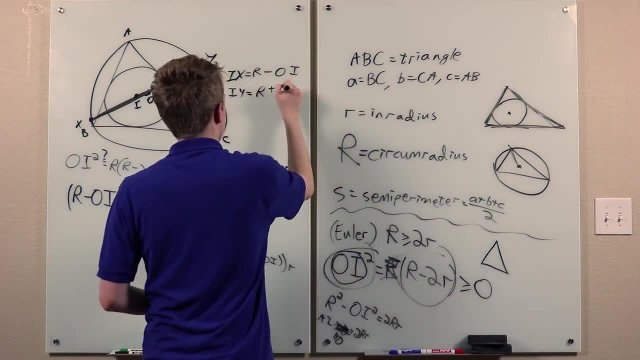 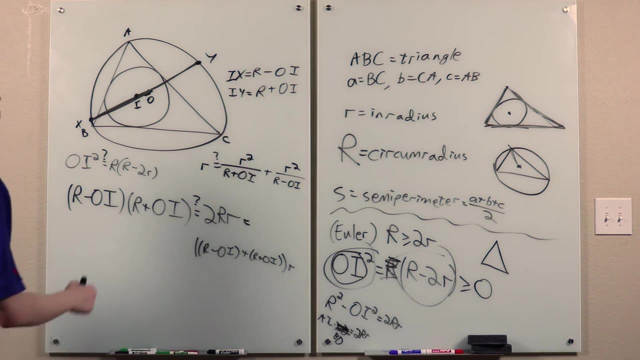 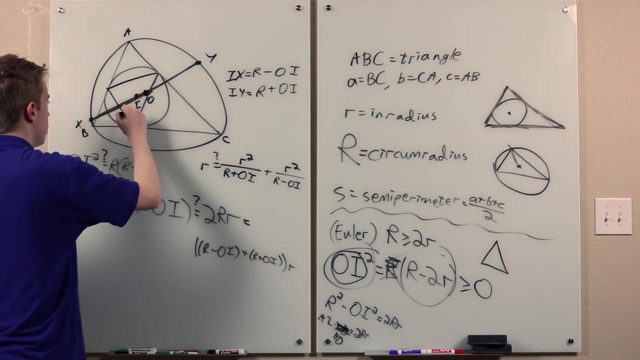 So if we invert about the in-circle, we know, we know that a, b, c, this- a inverts to the midpoint of this, b inverts to the midpoint of this and c inverts to the midpoint of this. 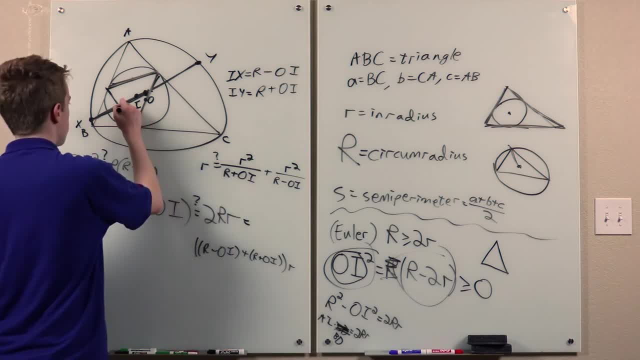 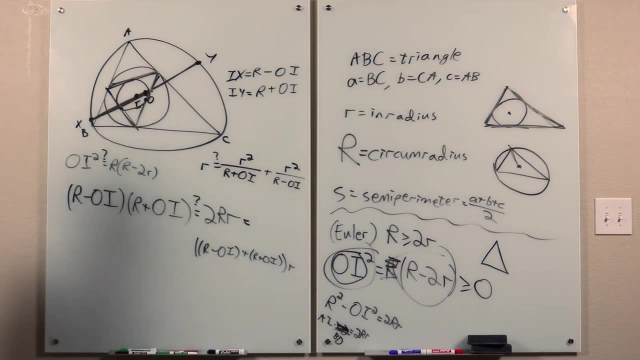 So the circumcircle of a, b, c will invert to the circle through these points, through these three points. So it's the circumcircle. so this will actually be the nine-point circle of the contact triangle, which is this, So the radius of this circle. 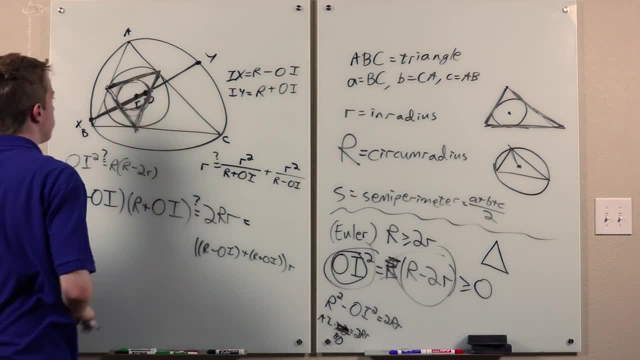 as, since it's the nine-point circle of this triangle, is half the radius. its radius is half of the radius of this, the circumcircle of the contact triangle. But that's just r the in-radius of a, b, c. 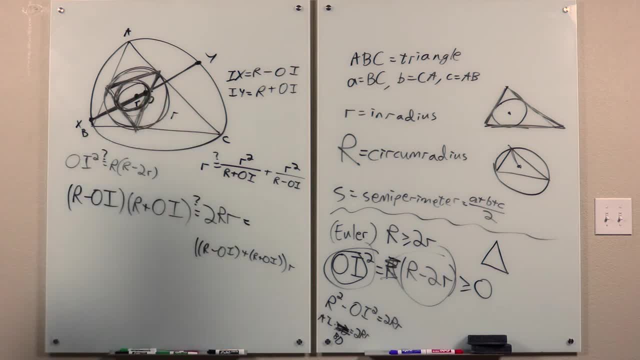 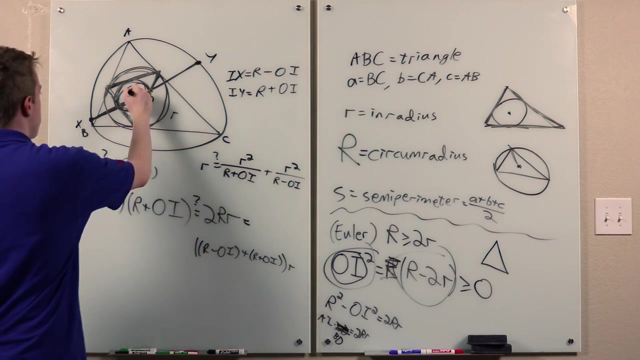 So this circle, its radius is r over two, so its diameter is little r. Now, furthermore, we notice that its circle must, no, its center must, lie somewhere on this line, Because, because i is the center of inversion, so the center of this circle, 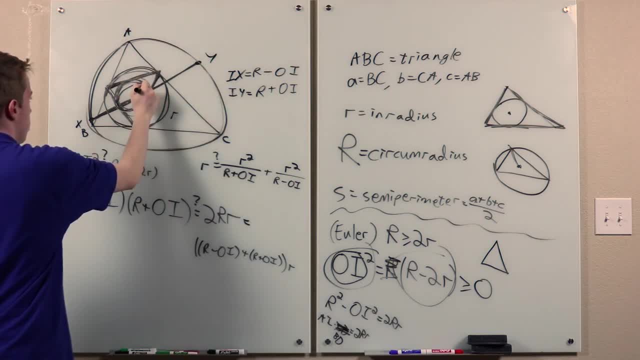 and the center of this circle, which is o the center of this circle and the center of this circle must be collinear with i. That's how. that's what happens with inversion, Like by symmetry, if we thought of it as a reflection over this line or something. 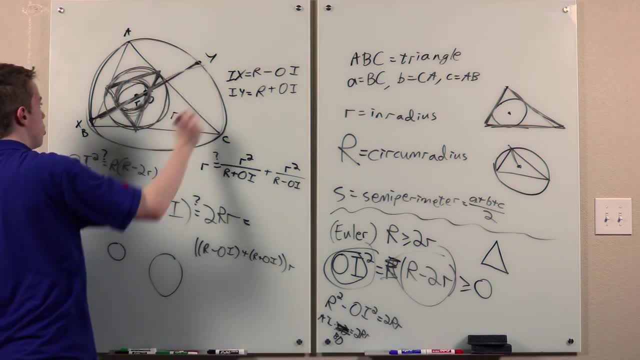 Then, like if we reflected over this line, this would stay the same, so this would have to stay the same, so its center lies on this line. Now look at the images of x and y. Call them x prime and y prime. 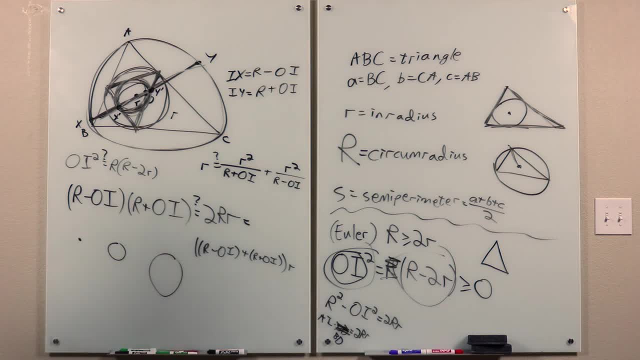 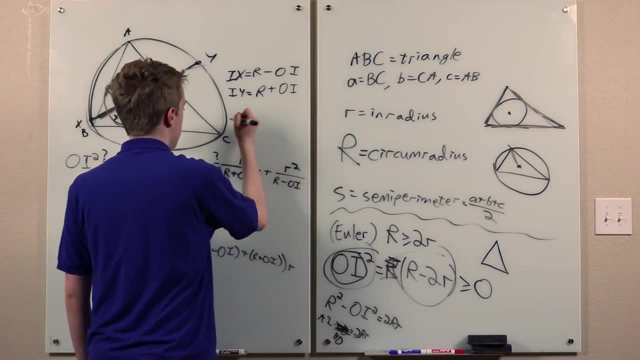 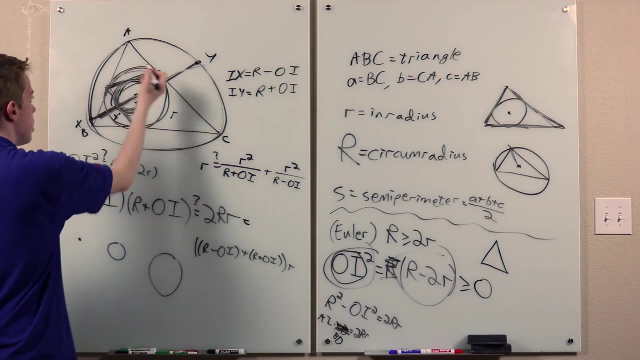 Then x? y passes through the center of this circle because it lies on this line. So x? y is a diameter of the of the circle, so its length is twice the radius, which is two times little r over two, Which is r. 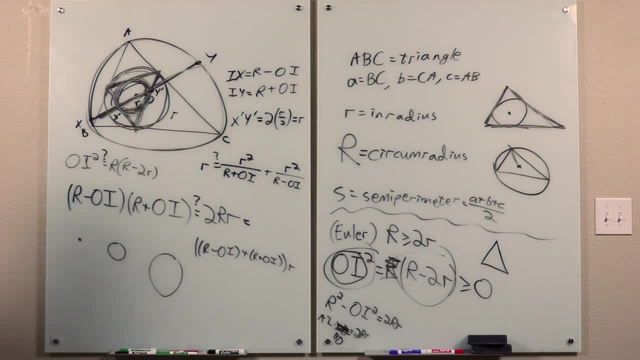 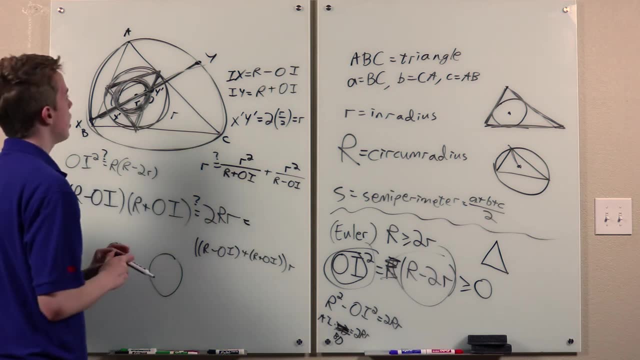 Now, um, uh, an easy little bit of angle chasing can show that this triangle is acute And from there we see that the its its circumcenter lying. so, like we can see, the eye lies inside this nine point circle. 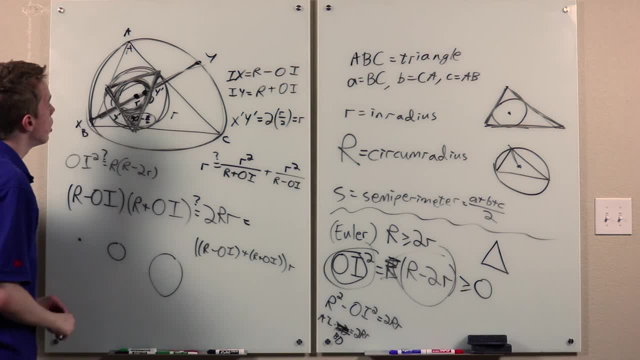 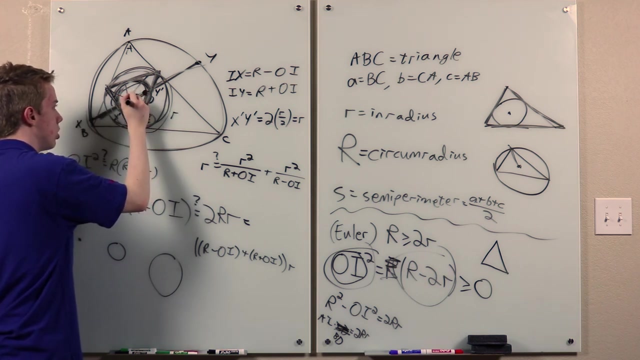 because the contact triangle is acute. Uh, so the circumcenter of the contact triangle lying inside the nine point circle, by homogeneity through its orthocenter, is equivalent to the reflection of the orthocenter of the of the contact triangle over the circumcenter of the contact triangle. 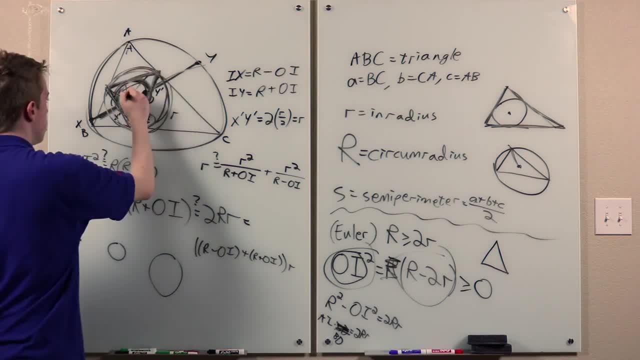 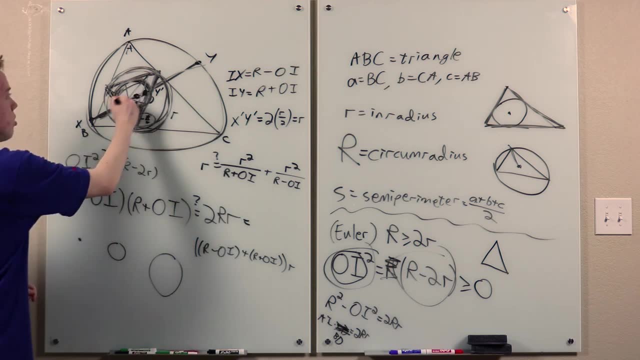 Being inside the circumcircle of the contact triangle, which is equivalent to the orthocenter of the contact triangle, lying inside the circumcircle, which we know happens since it's acute. So eye lies inside this nine point circle, meaning it lies on segment x, prime, y, prime. 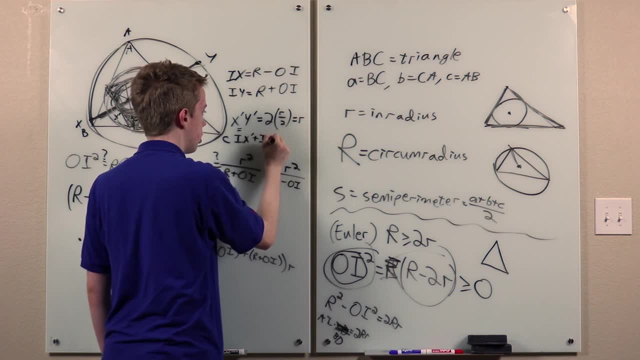 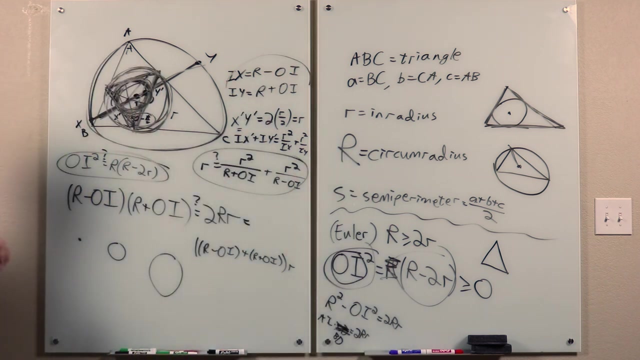 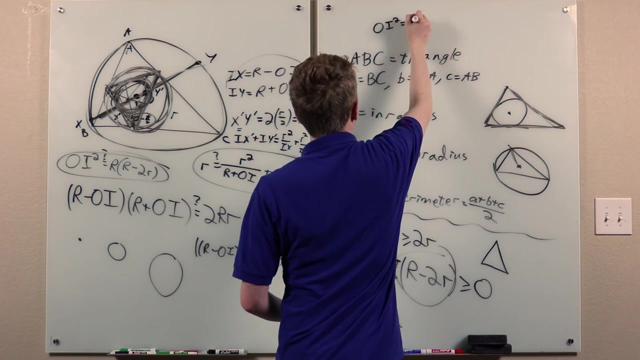 So we can write this as this, Which is exactly this, And we, from these, we get exactly what we wanted. We get this is true, and so we get this. So that proves this, And I'll want to keep this in mind for later.